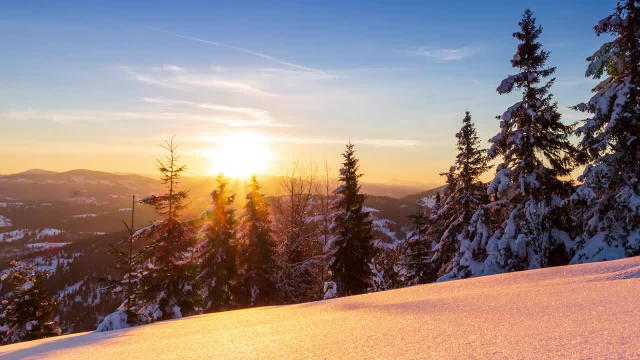 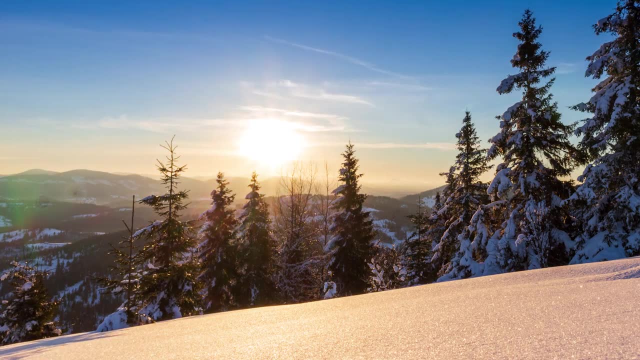 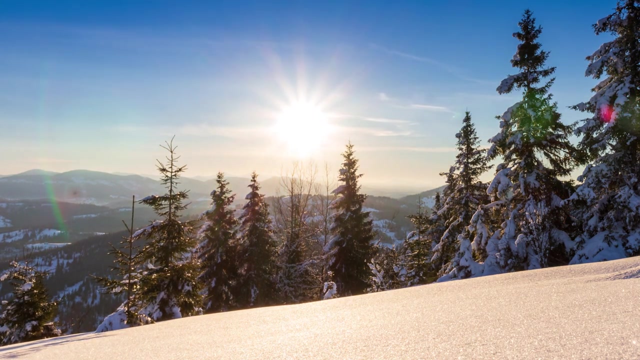 One of our most critical renewable resources is the sun. The energy from the sun heats our planet and, as we learned in our lessons on food chains and webs, it provides energy to almost every ecosystem on earth. Energy from the sun is a renewable resource because it's constantly being 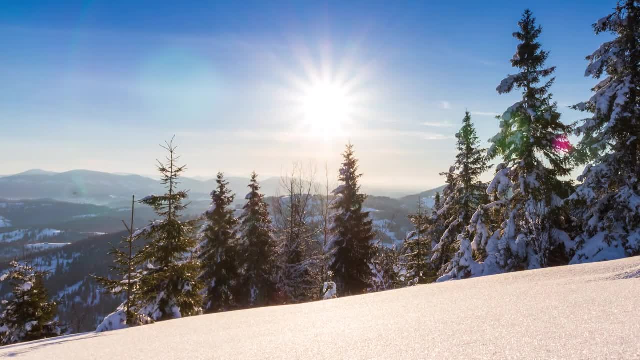 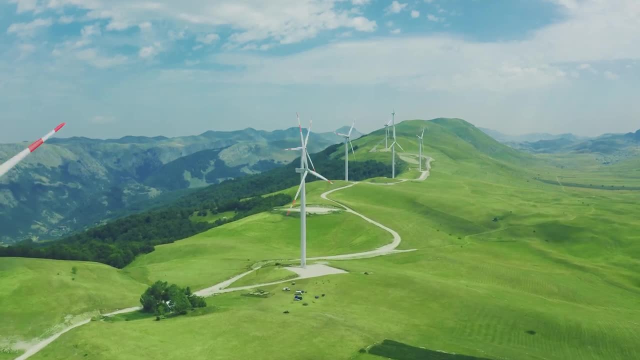 replaced. The sun will continue to emit less and less energy from the sun. The sun will continue to emit light and heat energy for billions of years, And as long as the sun is heating our planet, we'll also have wind, another key renewable resource. Wind is caused by differences in 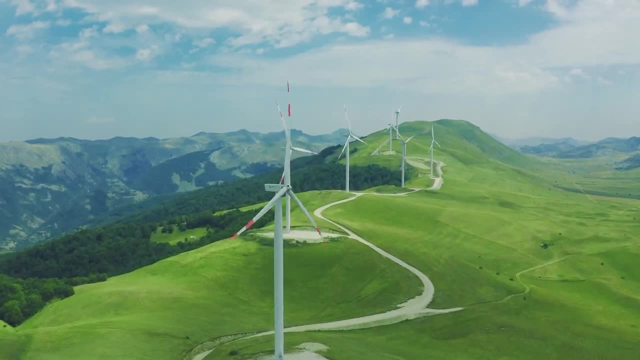 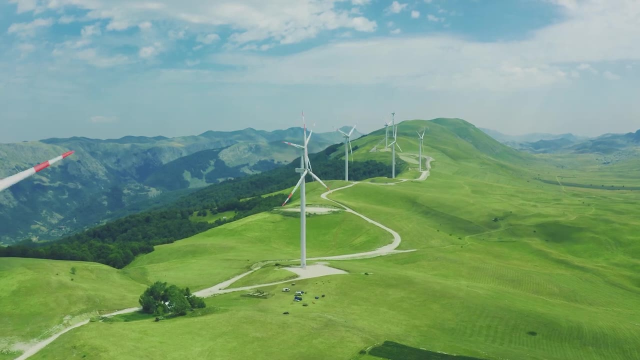 temperature in the atmosphere a result of the constant heating and cooling that happens during the day and night. Because of this, wind is constantly being generated, allowing us to use it to do tasks like turning windmills and turbines. Other resources are renewable because natural. 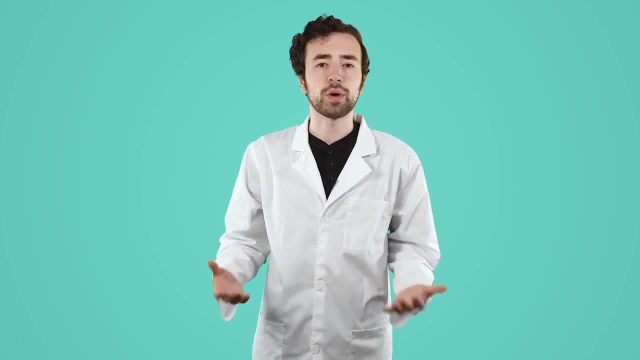 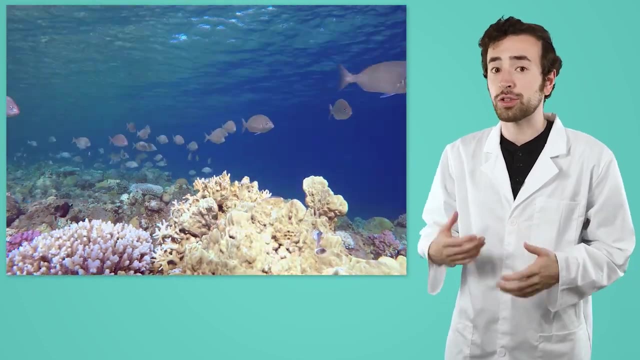 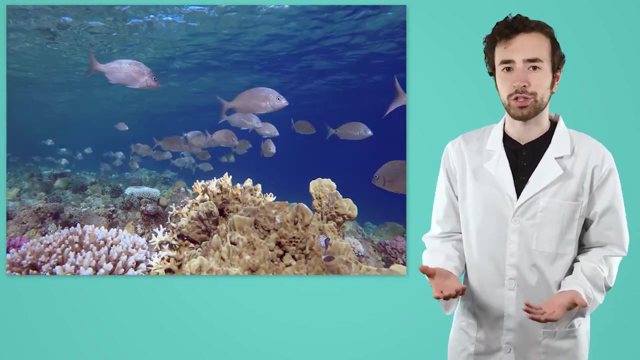 resources replace their supply as they're used. For example, animals that we eat for energy, such as fish, are a renewable resource. As we remove fish from the population to be eaten, more fish are born, replacing those that are removed. The population is replenished. 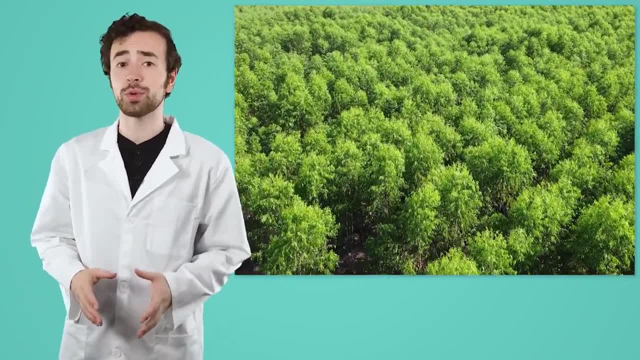 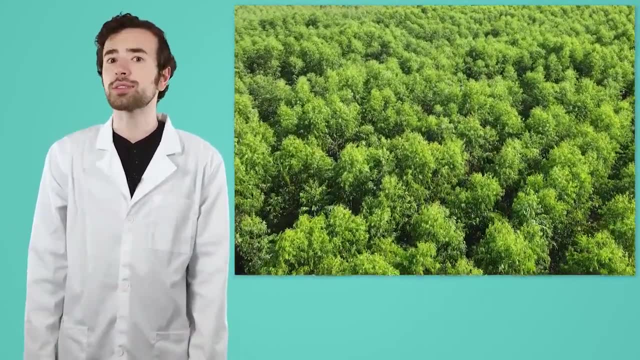 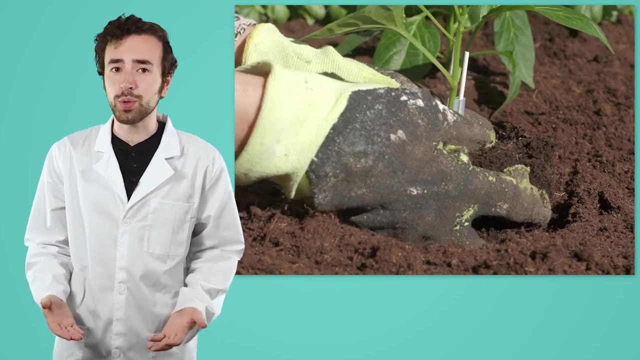 Trees are another extremely important renewable resource. We use trees for everything from building materials to cardboard to toilet paper. Trees are even used as a source of rubber, medicine and gum. We can ensure this important resource is renewable by replacing the trees we harvest with new trees and forests. While many natural resources are renewable, because they can be replaced as they're used, like animals and trees. others are renewable because their supply naturally cycles, like air and water. The nitrogen, oxygen and carbon dioxide in the air each cycle through the world's ecosystems, being used and replaced back. 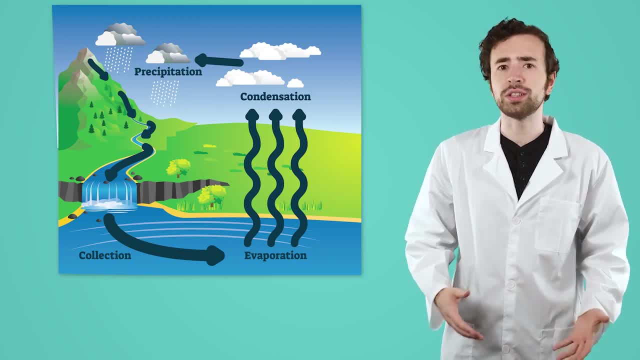 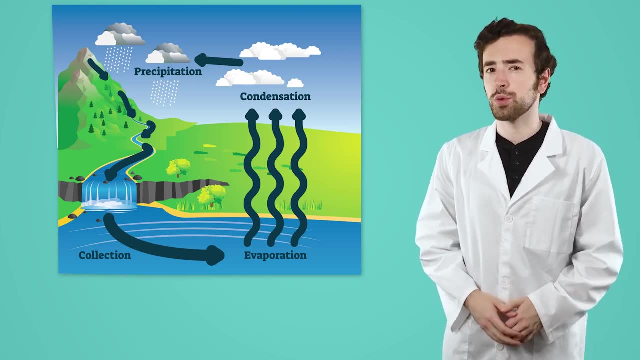 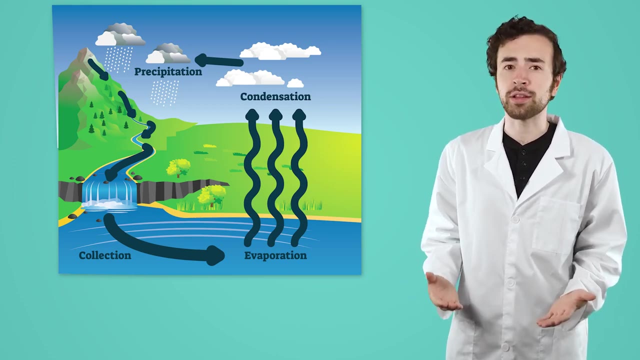 in the air. Similarly, water goes through the water cycle, continuously evaporating, condensing and precipitating. Replacing renewable resources and waiting for renewable resources to naturally cycle does take time, but not an extreme amount. They happen regularly and frequently enough to ensure these resources keep getting replenished. 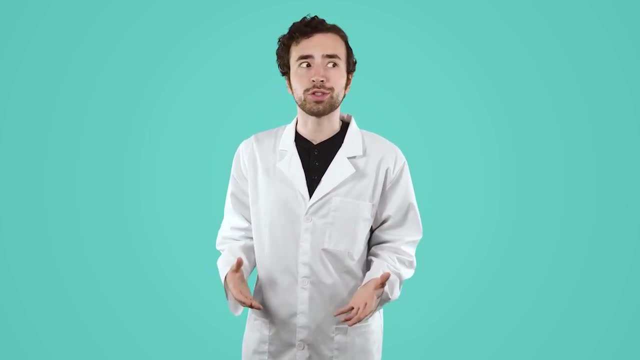 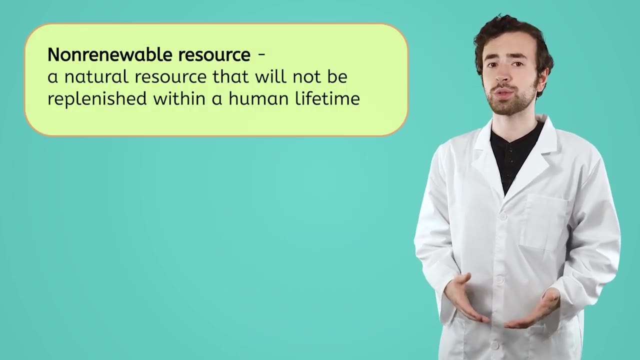 So renewable resources are ones that can be replenished relatively quickly. On the flip side, there are non-renewable resources. There are non-renewable resources that can be replenished quickly. A non-renewable resource is a natural resource that will not be replenished in our 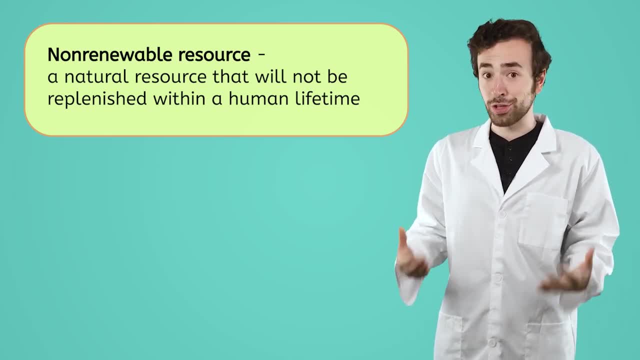 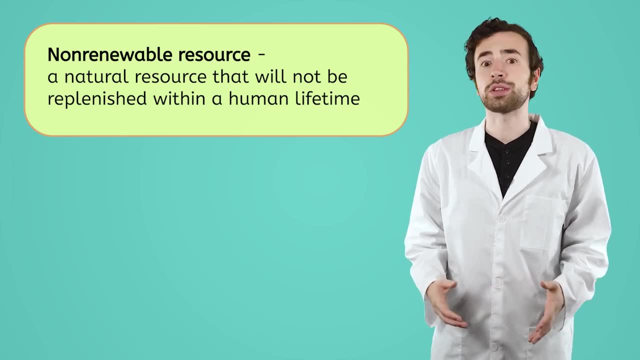 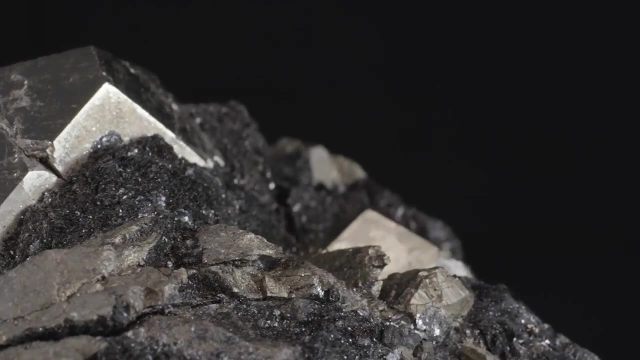 lifetimes, or even in many, many human lifetimes. Because non-renewable resources are used faster than they're replenished, there is a risk of them running out. Ore is an example of a non-renewable resource. It contains valuable minerals such as copper. 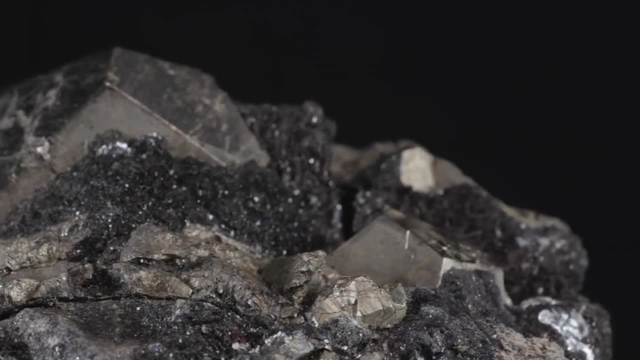 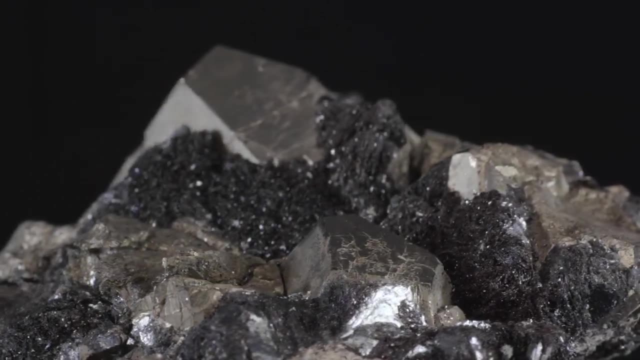 gold and iron, which are used in making everything from jewelry to electronics, to money and more. However, this ore is formed through the rock cycle, which is a process that can take thousands to millions of years. This makes it a non-renewable resource. 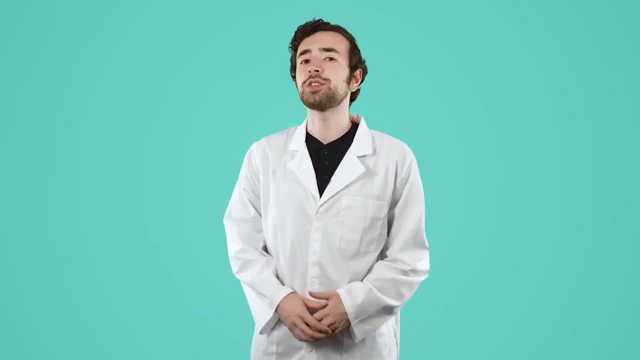 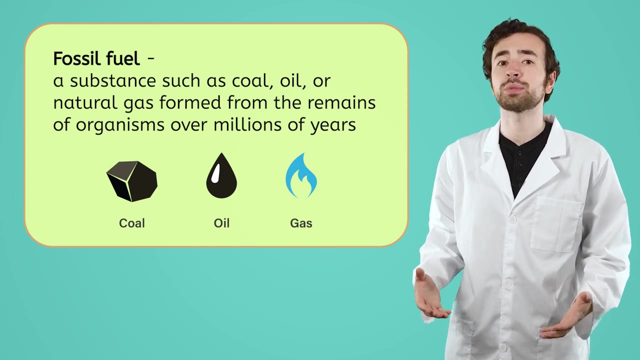 Often, when we're talking about non-renewable resources, we're referring to fossil fuels. These are things like coal, oil and natural gas that formed from the remains of organisms that lived millions of years ago Under extreme temperature and pressure. these remains became 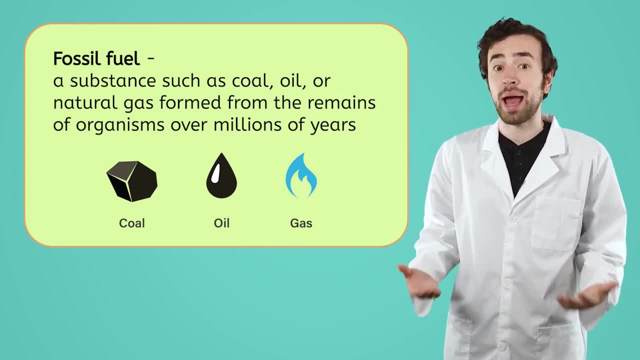 fossil fuels. This is a process that can take thousands to millions of years. This is a process that can take thousands of years. The energy from fossil fuels is what powers much of our world. We use fossil fuels to generate electricity, to fuel vehicles, to produce plastics and other. 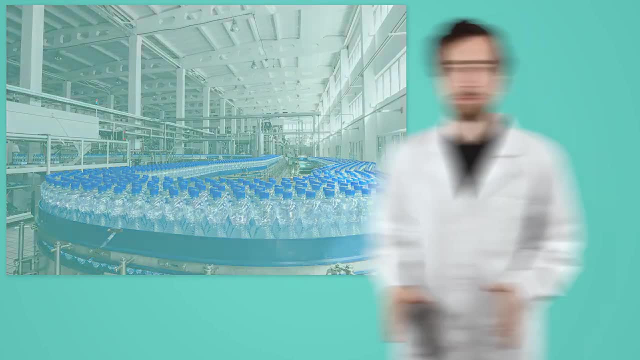 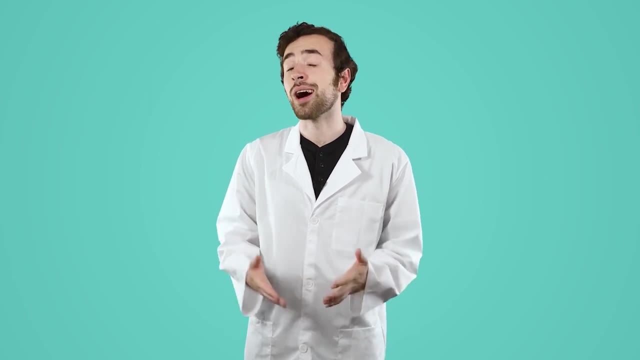 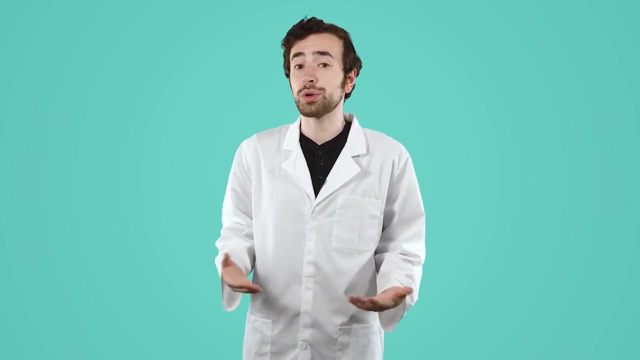 chemicals, and to do so so much more. But these resources are being used up much more quickly than new ones can form. That's why they're non-renewable. Fossil fuels aren't our only options for energy, though. Energy can be produced using renewable resources too: The energy from the sun. 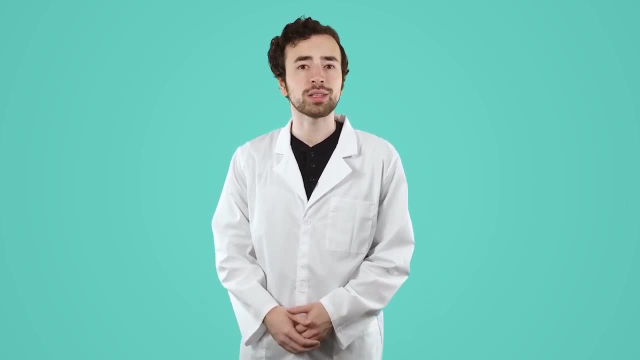 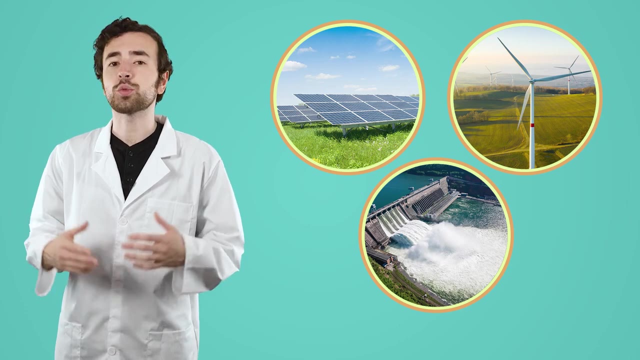 wind and the flow of water can all be used to produce electricity, using solar panels like the ones I'm installing on my house, wind turbines and hydropower technology. These renewable energy sources are more sustainable than burning fossil fuels and they produce less. 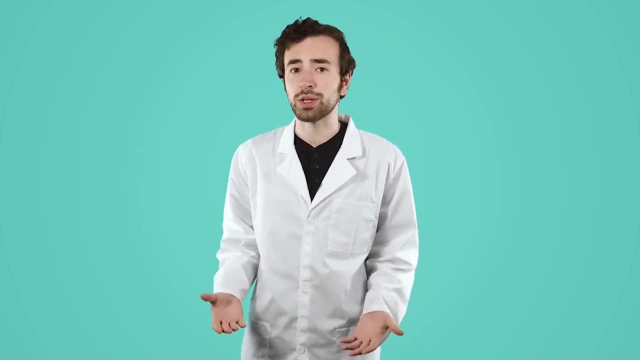 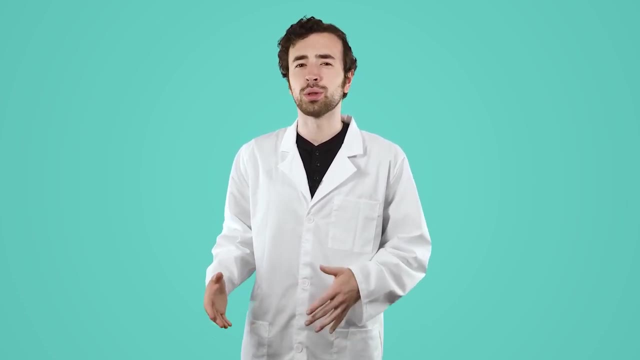 pollution too. But just like every other kind of resource, there are challenges to using renewable energy sources too. Can you think of what problems we might face in collecting solar, wind or hydropower? Pause the video here and record your. 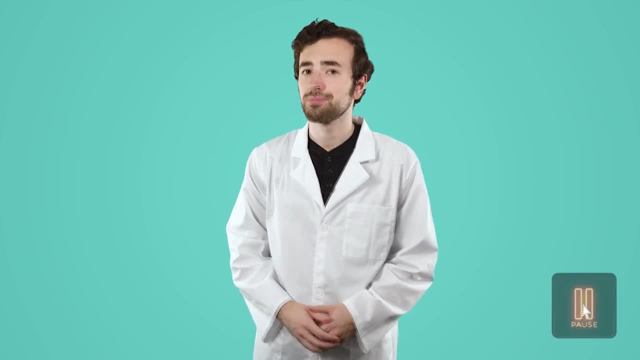 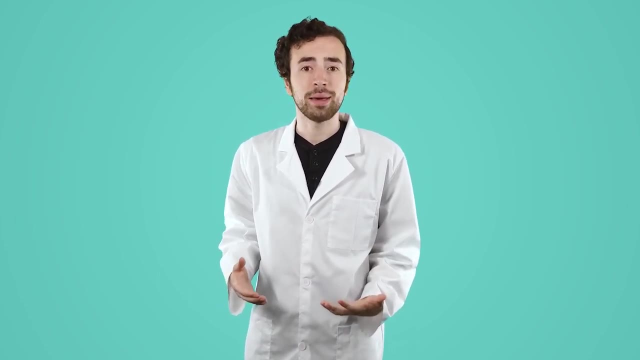 thoughts in your guided notes. Solar and wind energy are both weather-dependent, meaning they produce less energy on cloudy or windless days. Hydropower requires dams to generate electricity, which can disrupt ecosystems. Despite the challenges of renewable energy, scientists and engineers all over the world,